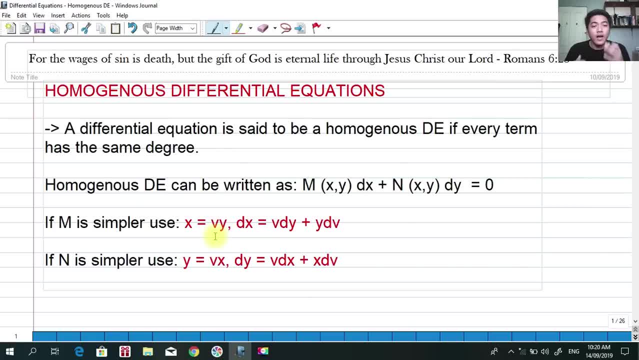 you use it because it would yield to another. if you use the other one, which is not simpler, it would yield to another integral, which is really hard to do. Okay, but you will still arrive at the same answer. Okay, if m is simpler, you're going to use this substitution. 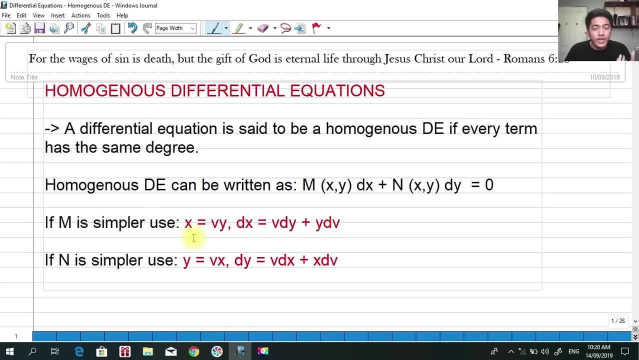 It's easy to memorize because if m is simpler, then x is equal to vy. If n is simpler, this function of n and n, as a function of x, of y we will be using, y is equal to vx. Then the derivative of dy is simply by product rule, again v, dx. copy the first and differentiate the second. 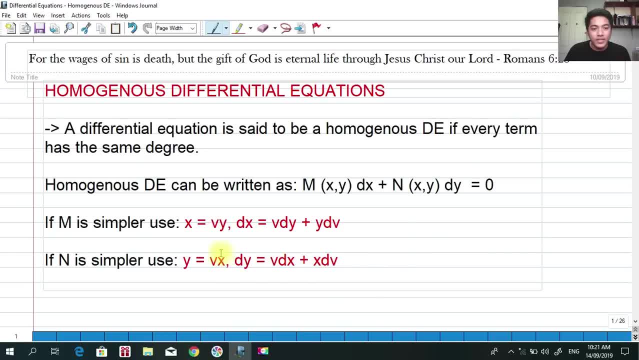 So that's why we have v dx, v dx here, plus again, copy the second x and differentiate the v So dv plus x dv So m is simpler, use this substitution. If n is simpler, use this substitution. Okay, so I advise you copy those formulas so that you would be able to not be lost in our topic. 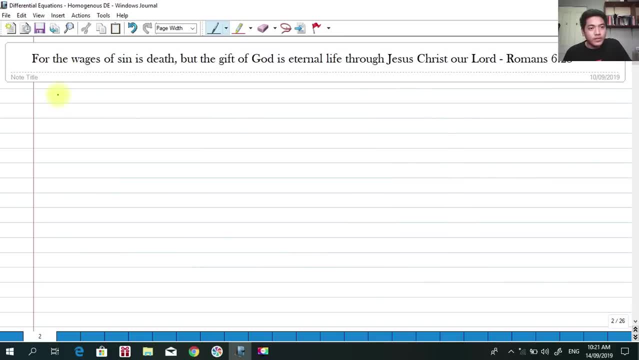 Okay. so for number one, we are basically solving the differential equation x squared minus xy- Okay, plus y squared. dx minus x, dy is equal to zero. So this is a homogeneous differential Because, as you can see, we have this term, X raised to two, x squared, which has a degree of two. 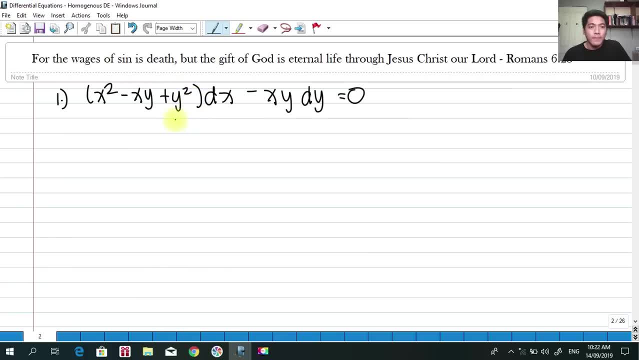 Okay, and also the y squared, which has a degree of 2.. And x- y. here, sir, why do we say that this is a homogeneous differential equation? Because the exponent of x is 1, the exponent of y is 1.. 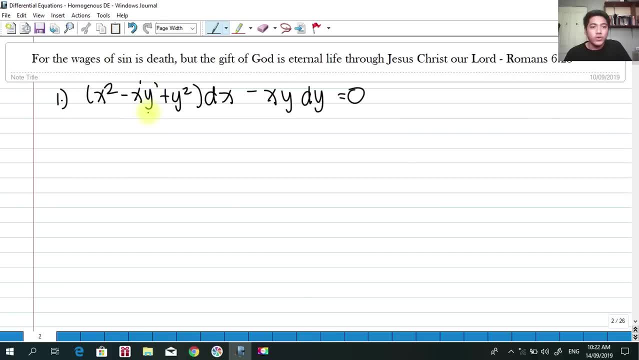 So if we add them together, since they are in multiplication, still this term, this whole term, has still a total degree of 2.. So hence, this is a degree of 2 for dx. So for dy, that is still the same. 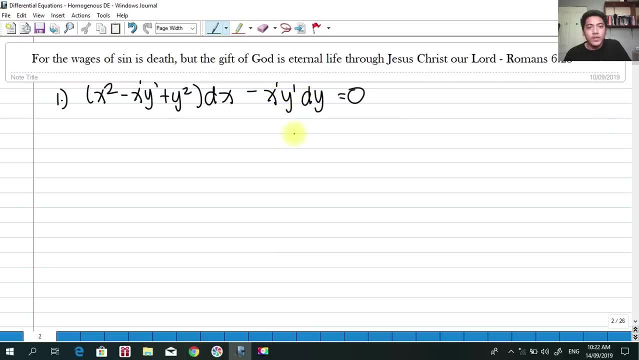 Since this has a degree of 1, still, if we add them, the total degree will be 2.. So this is a homogeneous differential equation with a degree of 2.. And we shall be labeling this as as what I have said a while ago. 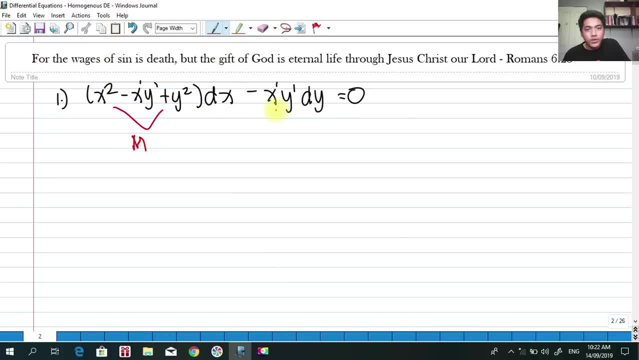 this term as the m and this term as the n. So, as you can see, here, m is a function of both x and y. n is a function of both x and y also. So in this case n is much simpler because it has x and y terms only, unlike this m. 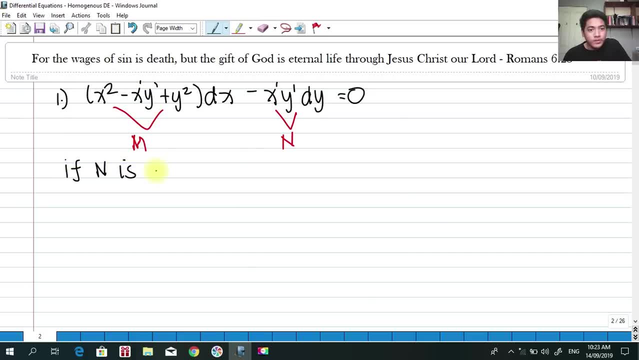 So if n is simpler, then we use the substitution let. y is equal to vx and then differentiate y So we have vdx plus xdv. So we're going to let these values Okay, Substituted in our original differential equation. 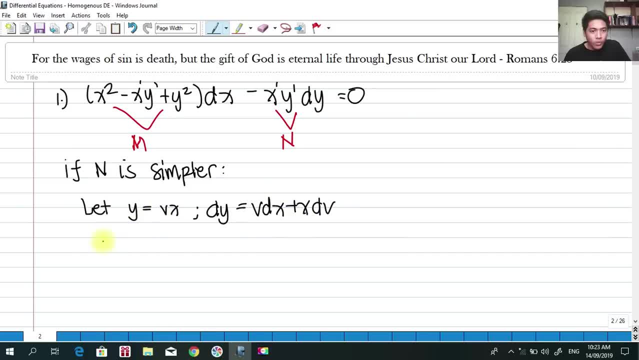 So if we let y is equal to vx and dy into this, what will happen is that we have x squared minus x times y. What is our y, vx plus y squared, which is vx squared? Then dx: okay, minus x times y. 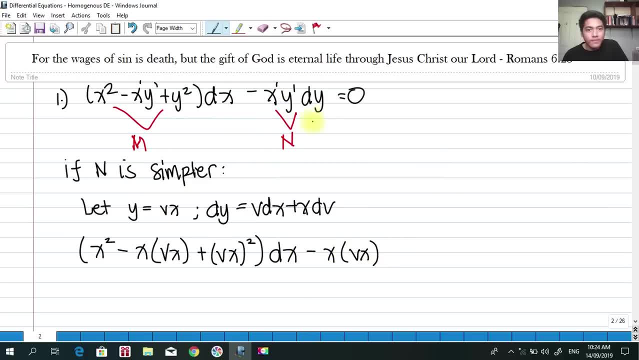 y. y is vx, Then we have dy, which is vdx plus xdv. So in other words, we simply substitute this simple substitution of y and dy into our original differential equation And from there we're going to simplify by algebra. 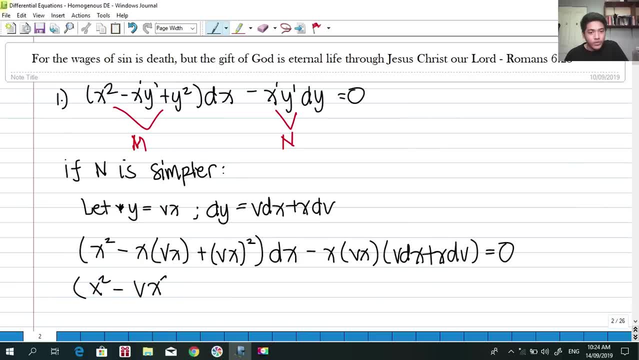 So we have x squared minus vx squared plus. this is raised to 2.. So we have v squared x squared, dx minus minus. I'm going to distribute this Minus. We have x or vx squared. Okay, We have vdx plus. xdv is equal to 0.. 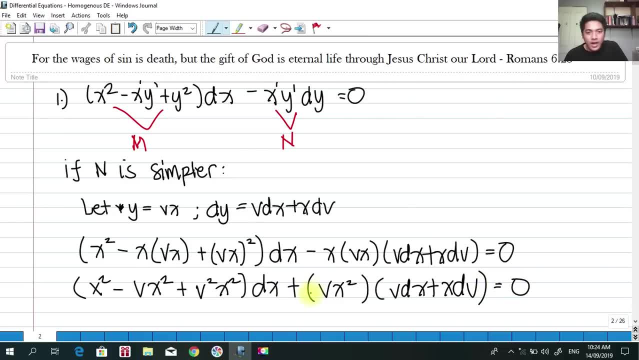 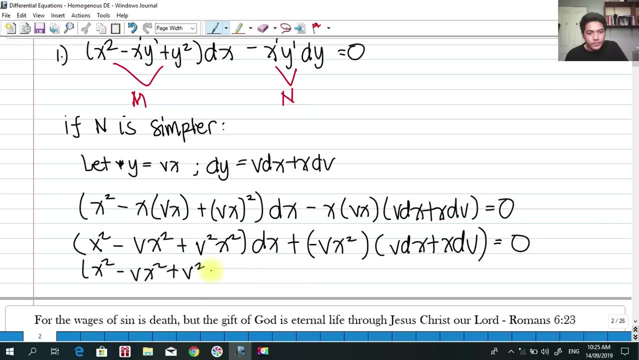 Okay, I can make this as a plus and I have a negative value here. Okay, That is still the same. Okay, So, furthermore, if you are going to so, for that, x squared minus vx squared plus v squared x squared dx. 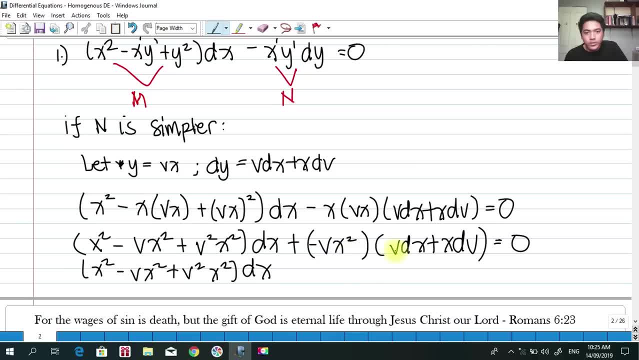 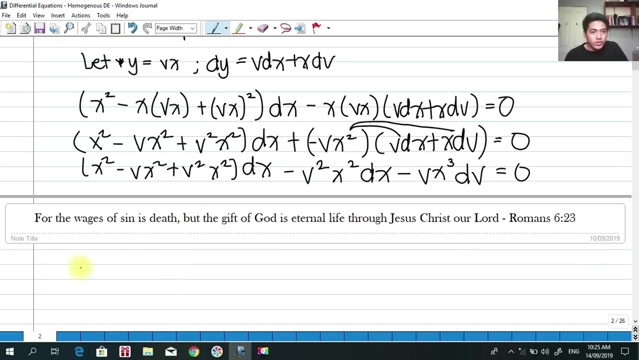 Okay, We're going to actually distribute this. So we have negative v squared: Okay. v squared x squared dx: Okay, Distribute this Okay. And then we have negative. what Negative vx? So we have negative vx squared dx minus vx squared dx plus v squared x squared dx. minus v squared x squared dx. minus vx squared dx minus vx squared dv is equal to 0.. 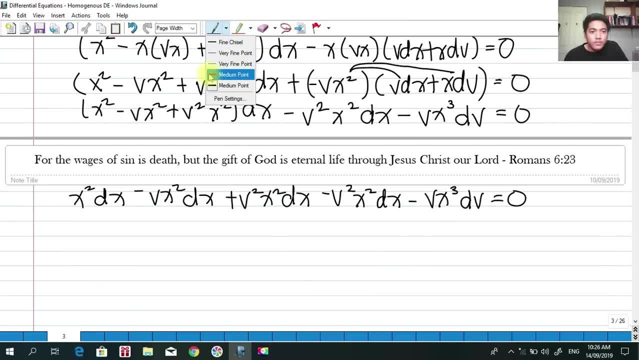 So, as you can see here we can calculate this. We can cancel out what this one: v squared x squared dx minus v squared x squared dx. All right, That should cancel out and we are left with: Okay, Can we still cancel out? 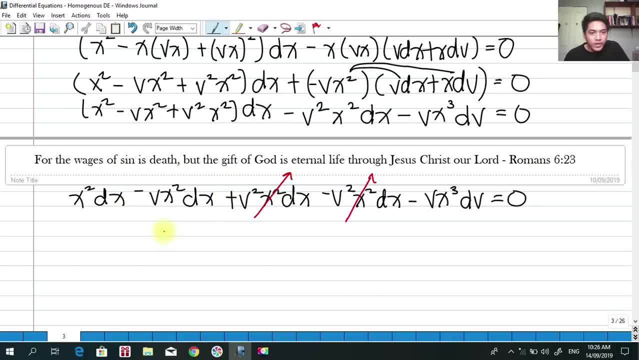 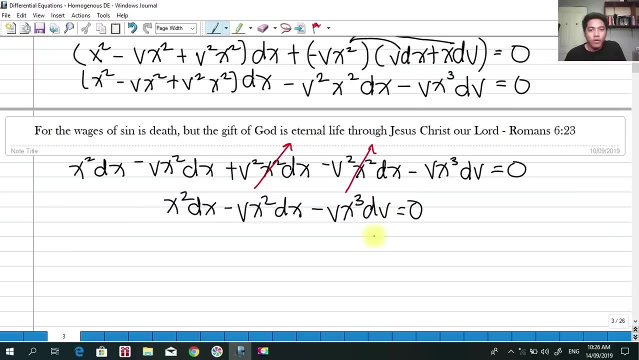 No x squared dx. So here's our answer. Okay, not not our answer, but the simplification of this. Okay, minus vx, cube dv is equal to Zero. Okay, So we should make this homogenous equation as simple as possible. 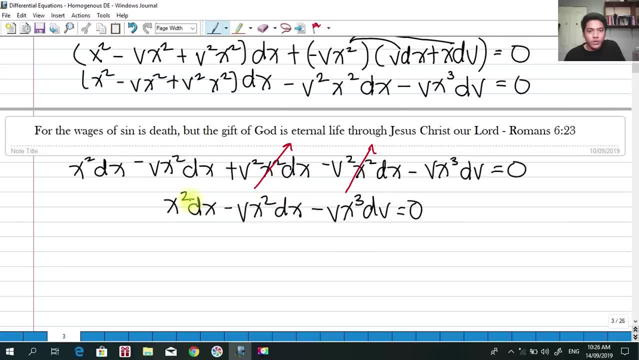 So, as you can see here in in this equation we have a common factor of x squared. So if I'm going to multiply this or divide all terms by x squared, what will happen? We will have be having dx here minus v dx. 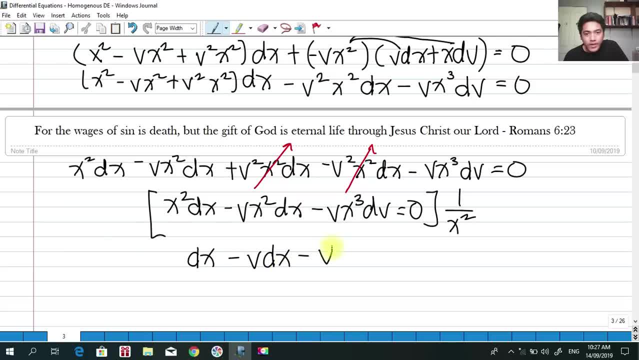 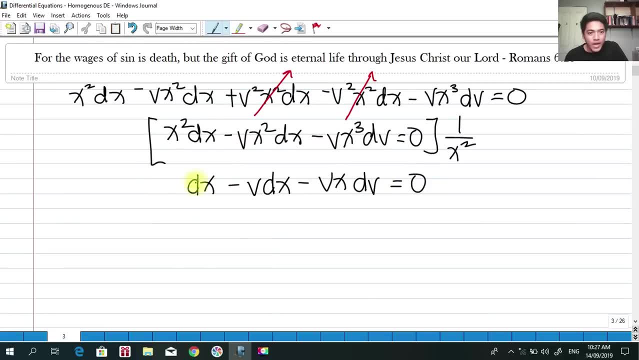 Okay, Minus vx dv is equal to 0.. So what are we going to do by like terms? So we have- I can factor out the x here- So we have 1 minus v dx, minus vx, Oops, minus vx dv. Okay. 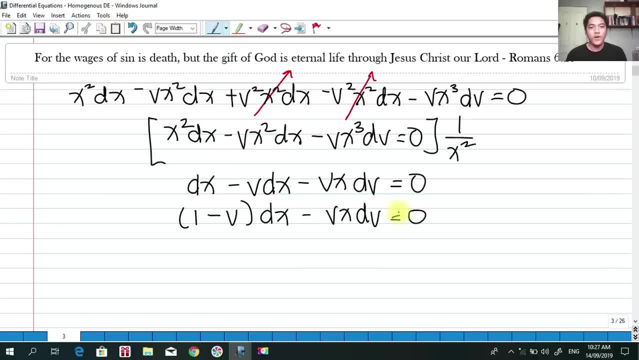 vx dv is equal to 0. So, as you can see here, this is a variable, separable equation. Okay, and if I'm going to again transpose this, on the other side of the equation, this becomes vx dv. So this is a variable, separable equation. 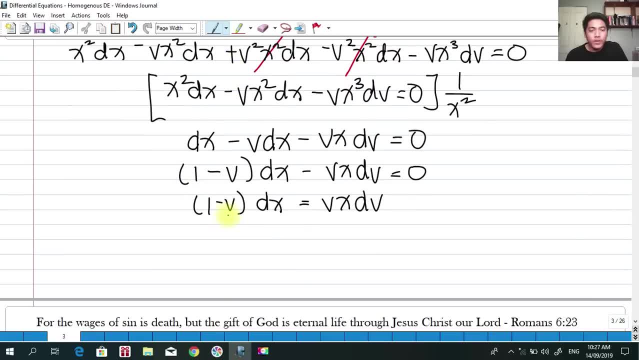 So we can now what: group all terms of v into dv and group all terms of x into x. So what will happen is that this is dx, This is dv. Okay, I need to eliminate this x on this term, on the this side of the equation. 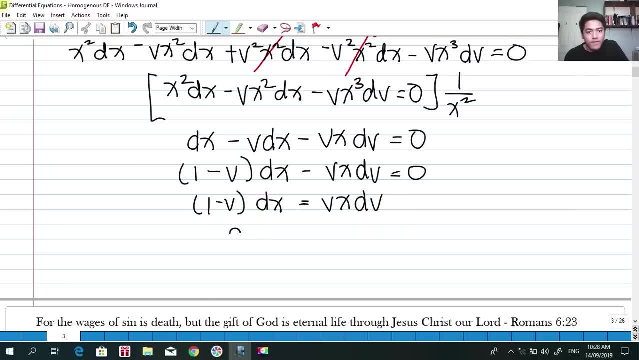 I'm going to eliminate 1 minus b on this side of the equation, So I have dx over this. x is equal now to v dv over 1 minus d. That is a variable separable equation. And what is the next step If you are able to arrange a variable separable equation into its corresponding dx and dv? 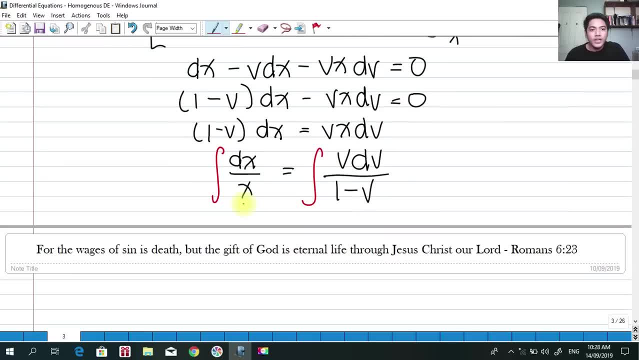 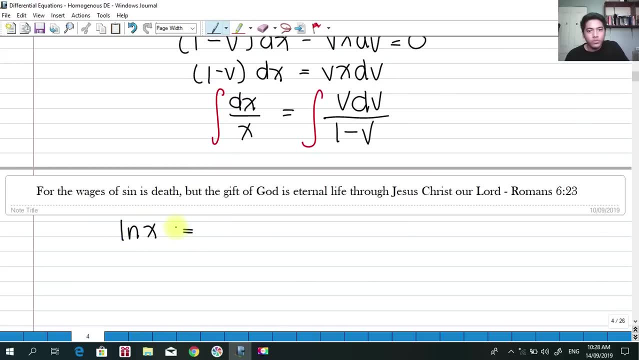 Okay, we have to integrate. Okay, upon integration. we know that integration of ln, x, dx over x is ln of x is equal now to: Okay, how do we integrate this? Now? my goal is to make this denominator the same as, or to make this numerator the same as the denominator. 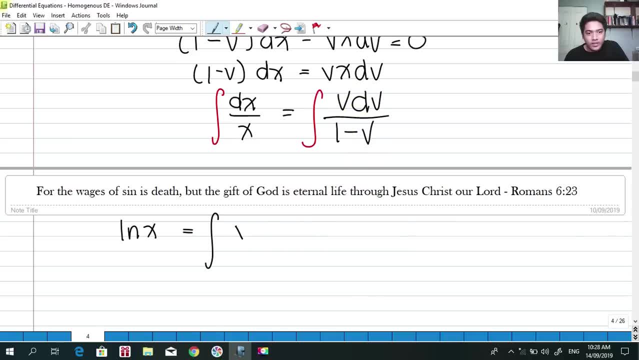 So if I'm going to rewrite the denominator or the numerator, I can rewrite this as this: v minus 1.. Okay, plus 1 over 1 minus v, dv. So this numerator is still the same as equal to v. Okay, if we, if we analyze this, v minus 1 plus 1 is still equal to v. 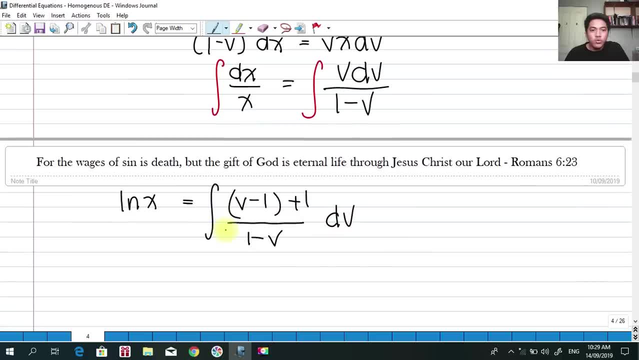 Okay. so the reason I did that is that we can use the properties of integral such that we can separate v minus 1 over 1 minus v, dv plus integral of dv, This is the 1 over 1 minus v. So if we're going to do that, ln of x. 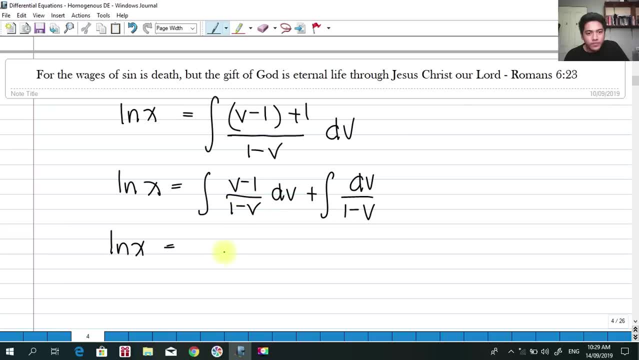 this is simply v minus 1.. Over 1 minus v. we can rewrite this as Okay. if we factor out the negative sign, we have 1 minus v here over 1 minus v. dv plus here. dv over 1 minus v. 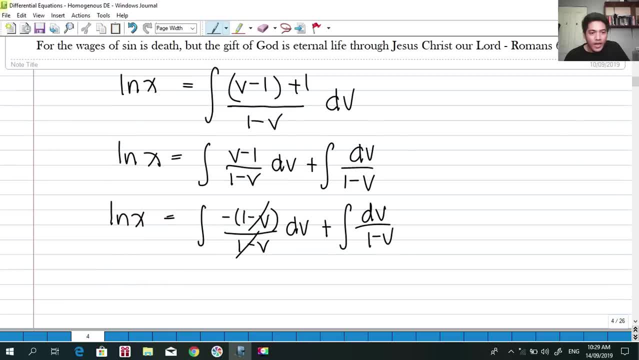 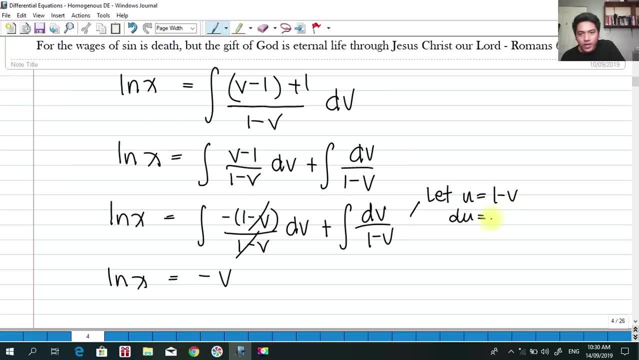 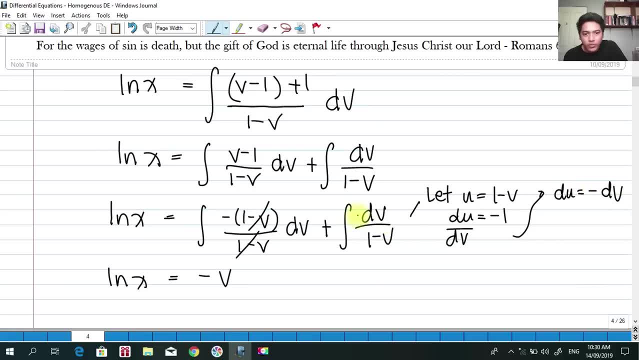 Okay so what will happen? Negative dv- I'm going to factor out negative dv here, negative 1 here and a correction factor of negative 1 here, So that we have negative ln of 1 minus v. Okay so, of course, 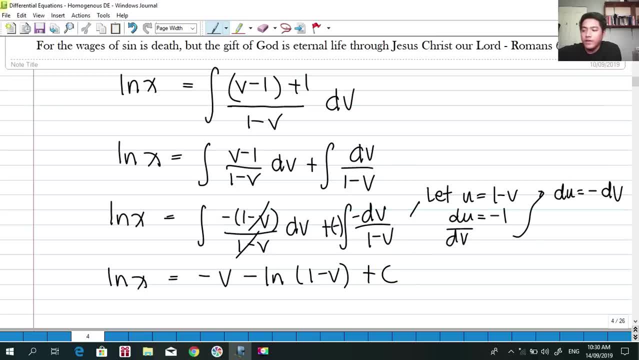 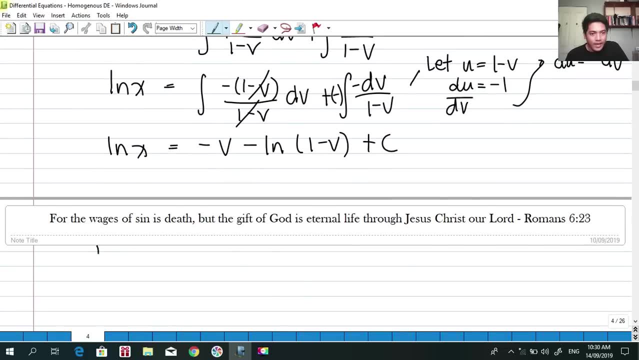 we have d plus c in here, Okay. so again, we're going to simplify that upon simplification. We have ln of x. Okay, ln of x plus v plus ln of 1 minus v is equals to c. Okay, that is equal to c. 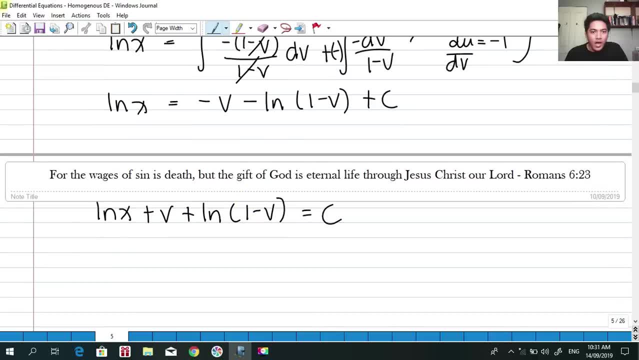 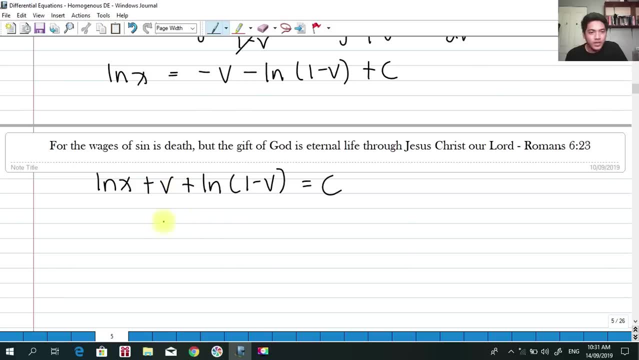 So what will I gonna do is to: I want to eliminate the ln. okay though I could not eliminate an ln here in our v-term, but still, if I'm going to exponentialize them, okay, exponentiate, okay, raised to something. 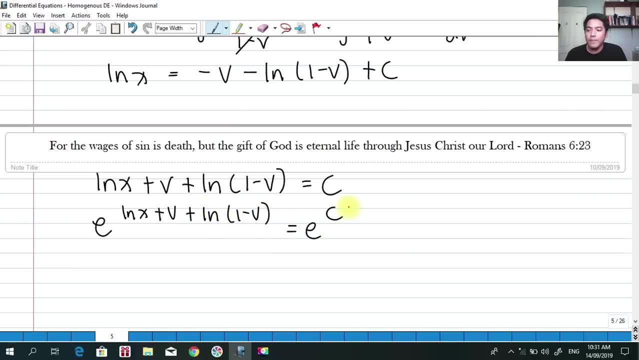 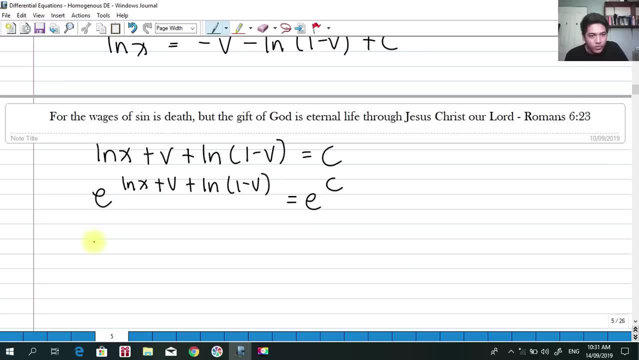 e. Okay, so we have e raised to c. So what will happen here? Okay, we know that this would be what. This would be equal to e raised to v Multiplied by e raised to ln of x plus ln of 1 minus v. 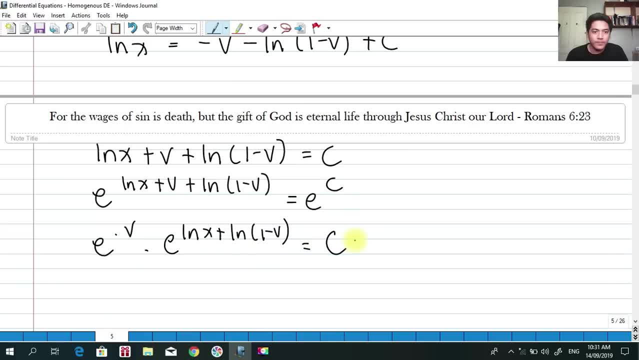 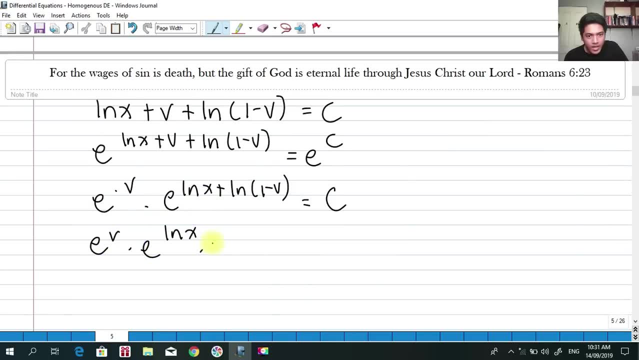 Okay, is equals to c, still c, Okay. and we know also that e raised to v plus e raised to ln of x times e raised to ln of 1 minus v- I forgot to actually rewrite this in terms of properties of exponents. 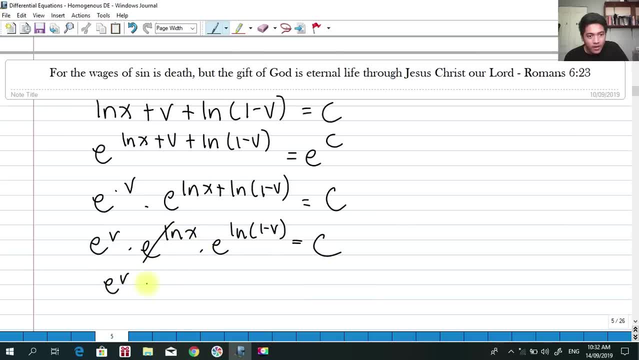 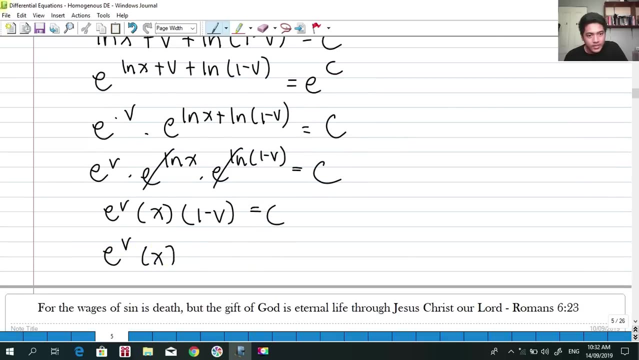 So we have e raised to v. so we have times x. e raised to ln of x with cancel e in ln, So we have 1 minus v here is equals to c. So in other words, we have e raised to v times x: 1 minus v is equals to c. 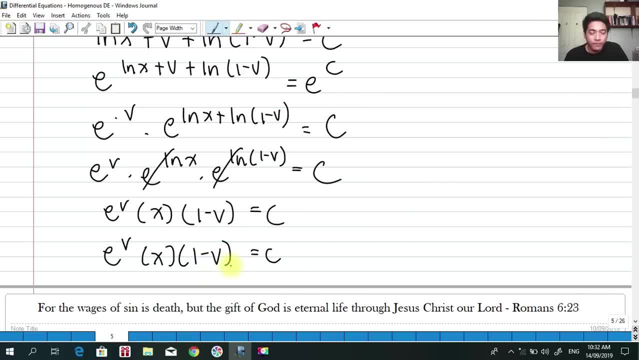 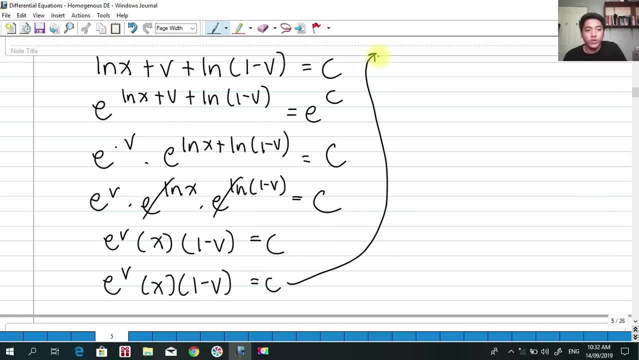 Okay, but our term here is v. Okay, we need to substitute back again the value of v into its original. Take note that we have a substitution a while ago: that y is equals to vx, So we need to get this in terms of v. 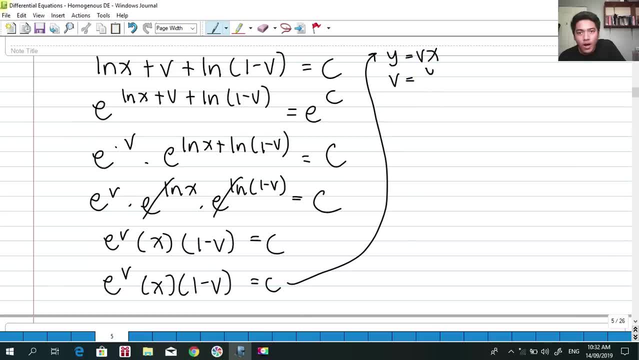 So v is equal now to y over x, And if we substitute that in our original, our equation, so we have now e raised to y over x, multiplied by x, multiplied by 1 minus v, which is y over x, is equals to c. 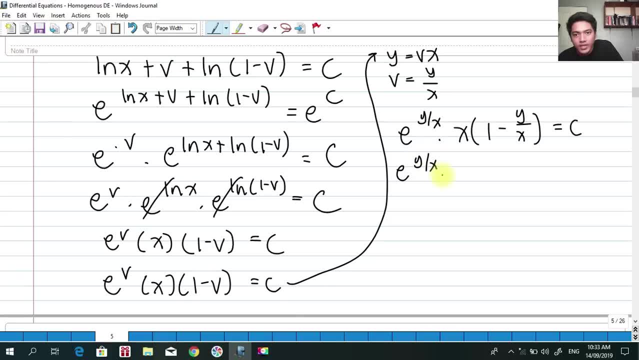 Okay. and if we further simplify this, e raised to y over x times x- Okay, this should be: x minus y over x is equals to c. We see here that x will cancel. So we are left with e raised to y over x times x minus y is equals to c. 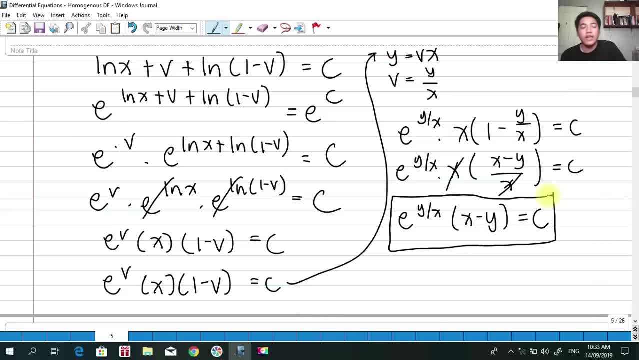 Now, this is our answer for solving that homogenous differential equation. Okay, so we need to substitute Back the v upon integration and upon simplifying these terms. Okay here, so that we could obtain the original differential equation. So let's try again. another example: 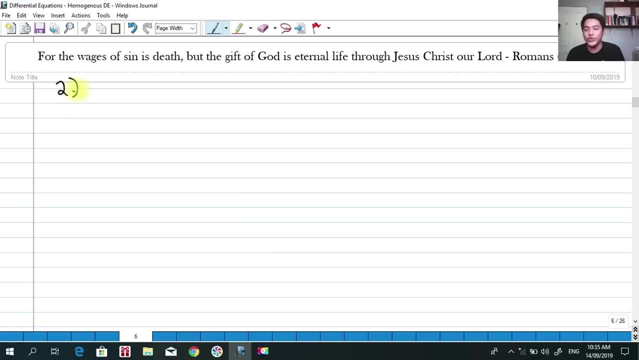 So for number two, as you can see, solving homogenous differential equation, it's a very lengthy process. Okay, so you have to recall your basics, all about algebra and integral Calculus and, of course, your differential, a little bit of your differential calculus. 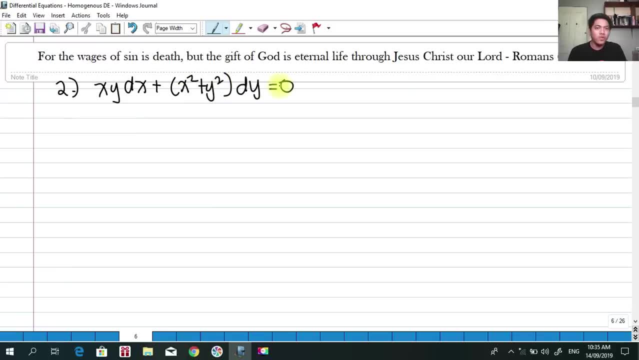 Okay, so here is our second example. So, as you can see, here we have this differential equation. This is a homogenous differential equation because each term has a degree of two. We have one here, one here If we add them. 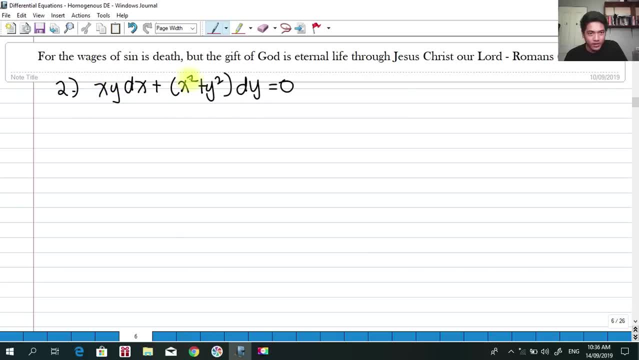 that is a total of two. This is another term with the degree of two, another term with the degree of two. Okay, again, this is m, This is n again, And what are we going to do here is to simply recognize which is more simpler. 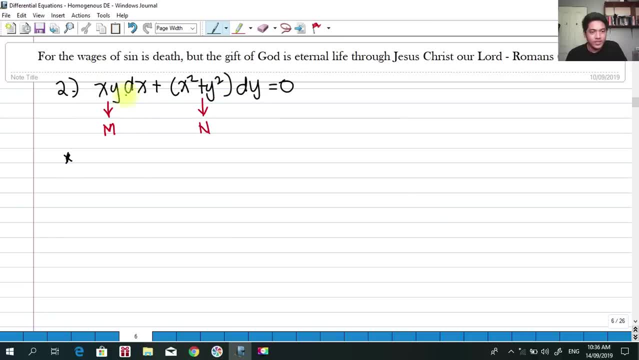 So in this case, our more simpler is m. this function Okay. so what are we going to do? if we let okay, x is equals to vy, because m is simpler, then our dx should be: dx is what vdy plus y. 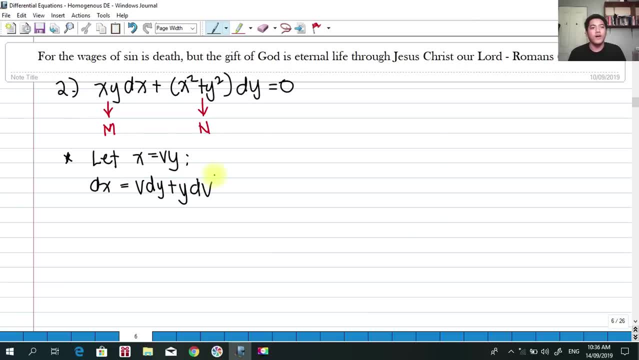 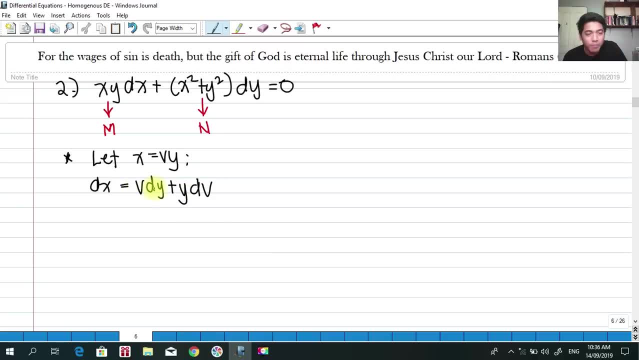 with this substitution, vy and all the values of dx with vdy plus ydv. So let's get started. So if you substitute it x to y, here we have vy multiplied by y. This is x multiplied by y, And our dx is simply vdy plus ydv. 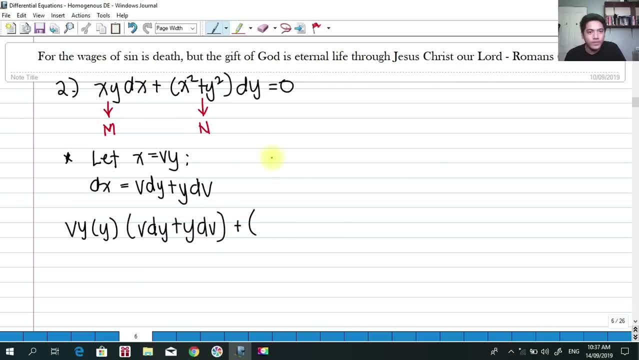 that is our dx, Plus, of course we have x squared, So can I rewrite it as b squared, y squared already, already right, because uh, this is raised to two. so plus y squared, okay, times dy is equals to zero. so if i'm going to pack, uh, uh, i mean we're going to. 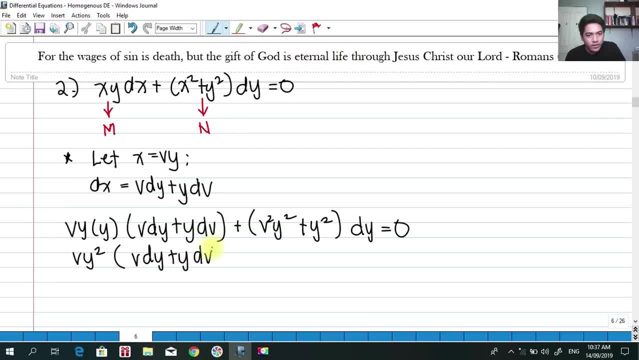 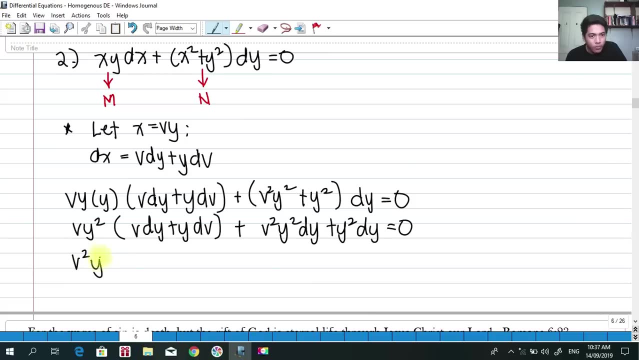 simplify this: bdy plus ydb- okay. plus we have b squared y. squared dy plus y squared dy is equals to zero and uh distribute this: okay, so we have b squared y squared. okay, let me just uh rewrite this: b squared y squared dy, okay. by squared times ydb. that should become by u. 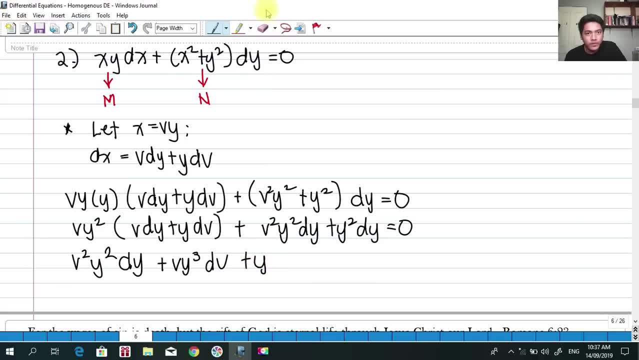 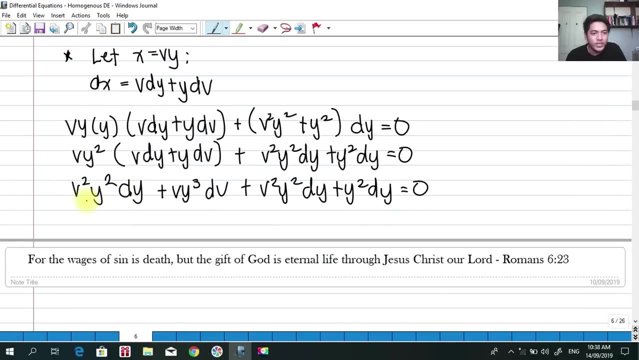 dv plus v, oops, plus v squared ydb y squared dy plus y squared dy is equals to zero. can we simplify? okay, as you can see, here we have b y squared d y, b squared y squared dy. we have b squared y squared dy. here we can add them, so we: 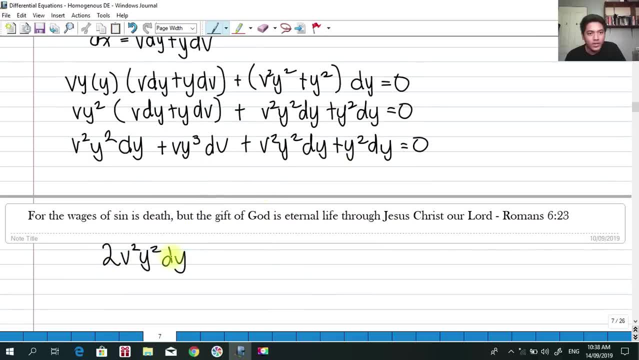 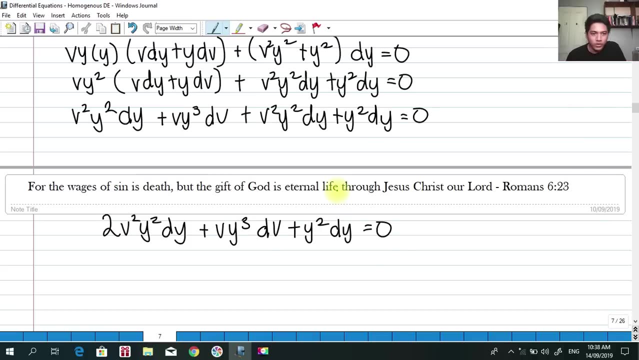 have two b squared, y squared dy, and we can copy the other, vy cube dv, this one and this one plus y squared dy is equals to zero. so do they have common factors? do each term here have a common factor? yes, we can actually divide them. we have y squared here. we can strip off y squared here and we have y squared here. so 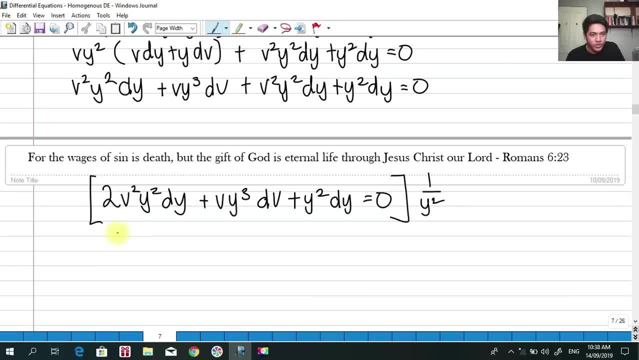 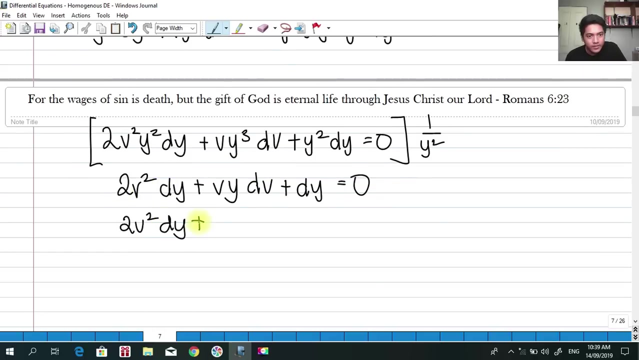 we can divide the whole side of the equation by y squared so that we have 2b squared. okay, dy plus vy, dv, because the y squared here will cancel out. so we have a remaining of y because up. so i can factor out d, y. so to b squared plus one, we have 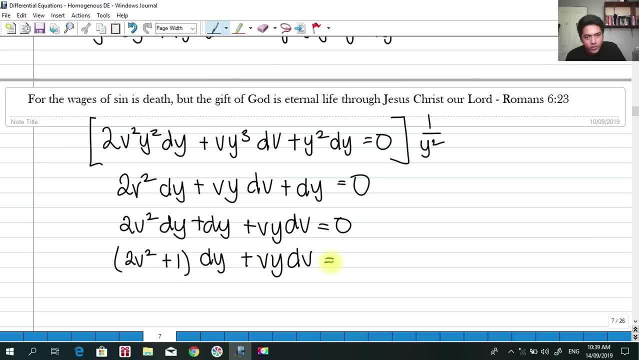 dy here plus by dv is equal to zero. so now tell me, is this a variable separable equation? so let's look at: loosen for b by dy, with magnitude plus b, and then my formula is simple: dy is equal to zero. so, combining like terms, let's just do this and then so we have, we have, we can have this. okay. so i can factor out d, y, so i can factor out by. so 2v squared plus 1, we have dy here plus py, b is equals to zero, okay. so now tell me, is this a variable separable equation? okay, is this a variable separable equation? o. 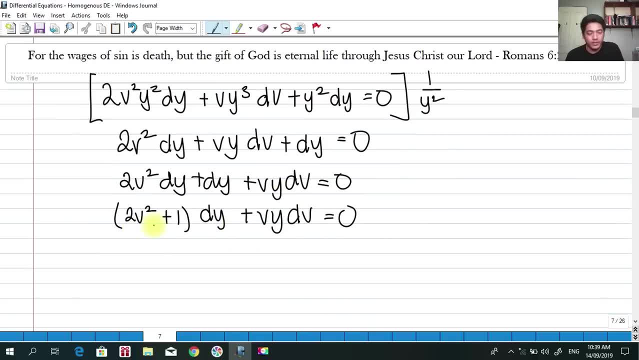 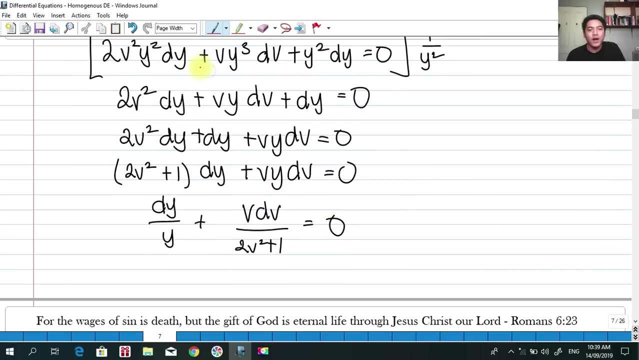 o parable. Yes, that is So. if I'm going to rearrange this, this should be: dy over y plus vdv over 2v squared plus 1 is equals to 0.. Okay, so what's the next step After arranging this variable? 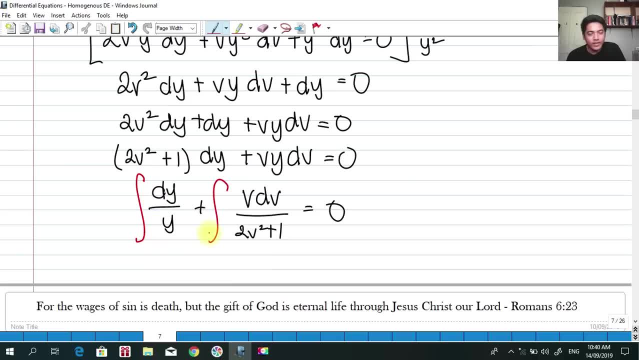 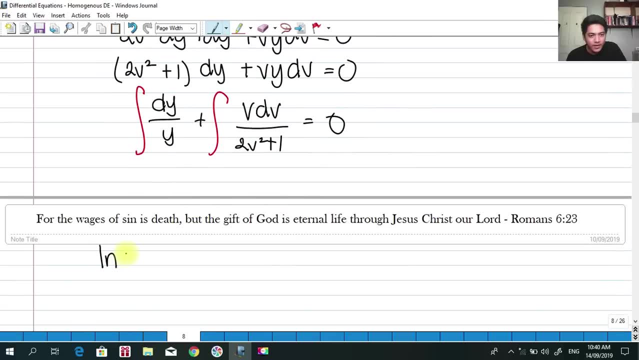 separable again, we need to integrate both sides. So upon integration, we know that dy over y, that's the easiest one. We have the ln of y Plus. let me just rewrite this vdv: over 2v squared. 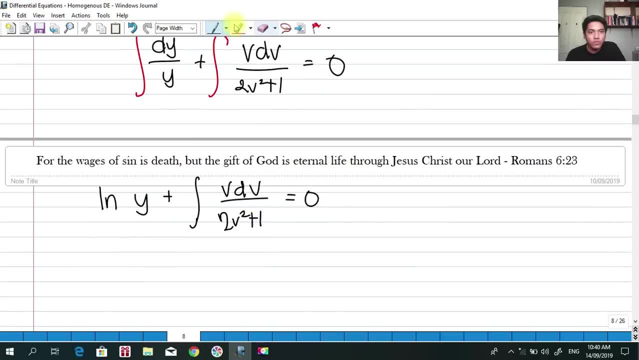 plus 1 is equals to 0.. So if we let now, okay, if we let now let u, as 2v squared plus 1, with respect to v, is 4v dv, of which this vdv vdv is available on our integral, But we have a 4. 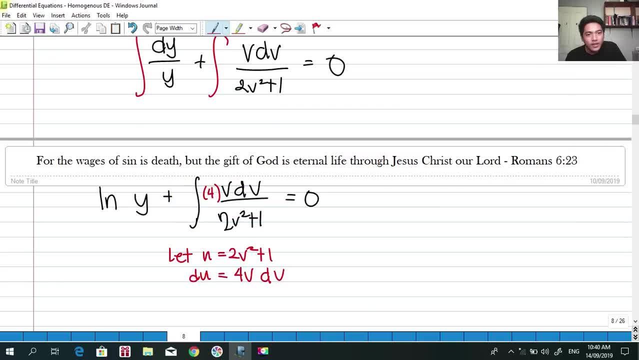 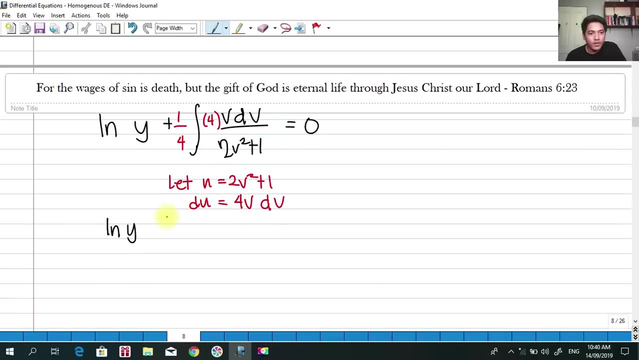 here. So you have to offset a 4 here and correction factor outside of the integral of 1, 4.. Okay, because just to have a u substitution here. So what will happen here is that we have an ln of y plus 1, 4.. 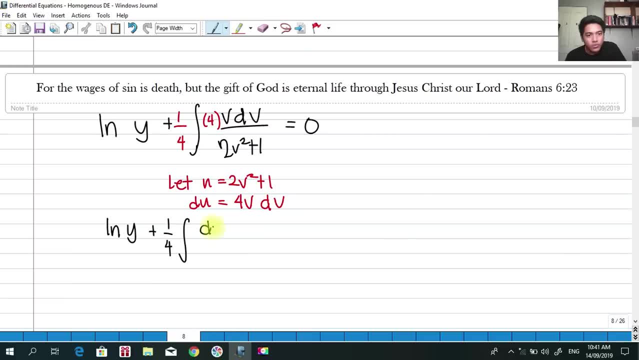 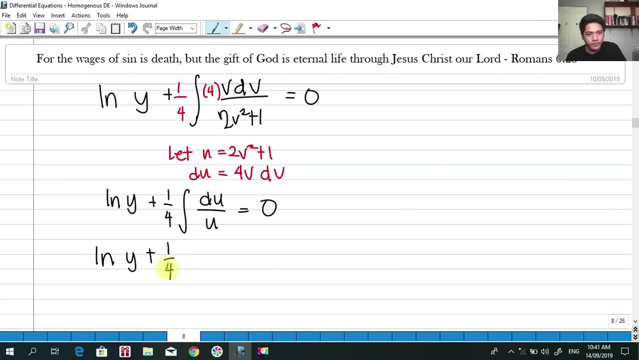 The integral of 4vdv is du over. u is equals to 0.. Okay, so if we integrate that ln of y plus 1, 4.. Okay, ln of u, this would be ln of u, but u is equal to 2v squared plus 1.. Now we integrate: 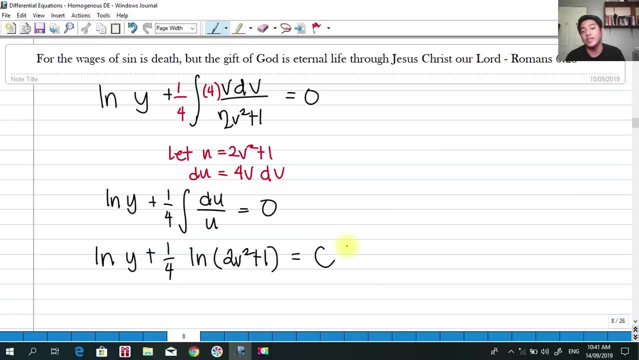 both sides here. So we have, we can write a constant here, Okay. so it's okay. it's always necessary to write a constant Whenever you do integrals. So it's okay also to write here in the right side. So, most commonly, 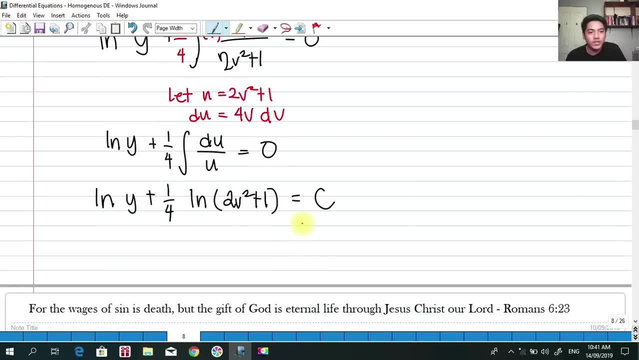 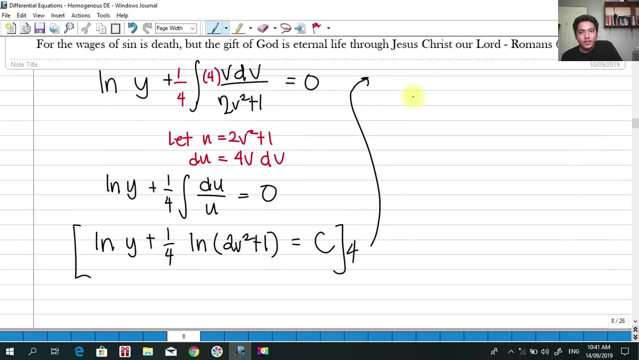 it is being written on the right side. So we have now this result. Okay, so let's first simplify before we eliminate the ln, If I'm going to multiply both sides of the equation by 4, so what will happen is that this should become 4 ln of y plus ln of 2v squared. 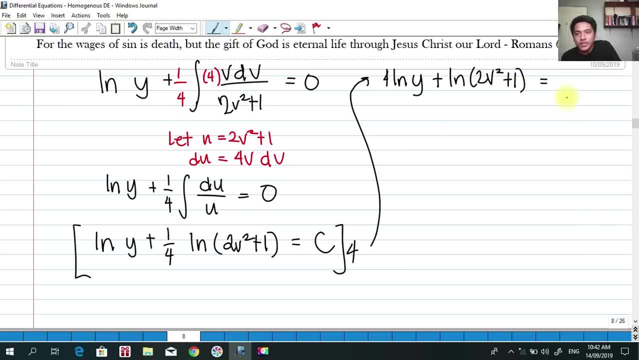 Plus 1 is equal to 4 times a constant is still a constant. that should be still a constant. If this is a variable, if you multiply it by a variable, then you should include the variable. Okay, so we have by properties of ln, we can rewrite this as ln y raised to 4,. 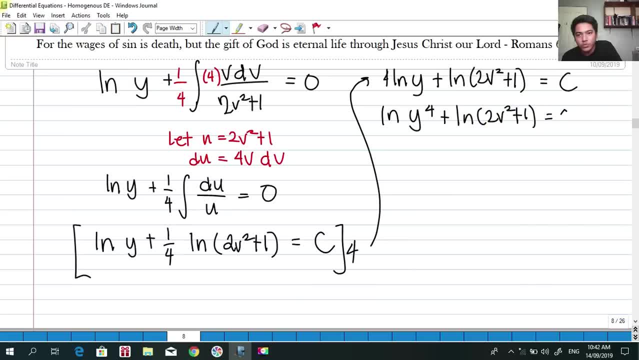 plus ln. 2v squared plus 1, is equals to C and of course we can rewrite this. properties of ln. We have ln y raised to 4, raised to 4, multiplied by 2b squared plus 1 is equals to C, and if we are: 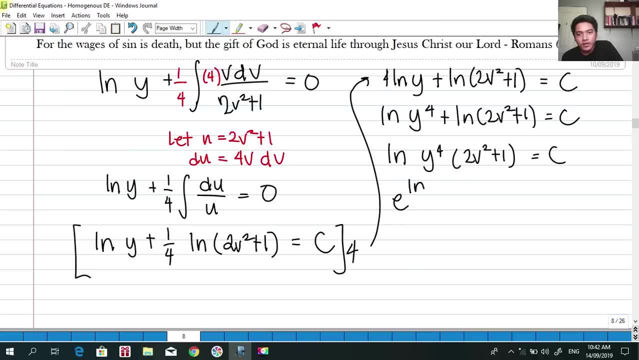 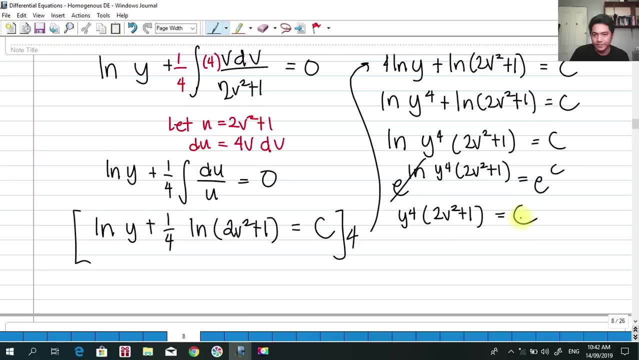 going to eliminate that and we must exponentiate: okay, y raised to 4, 2b squared plus 1 is equals to e raised to C, so we can see that this would cancel. so we are left with y raised to 4. 2b squared plus 1 is equals to still C, okay. 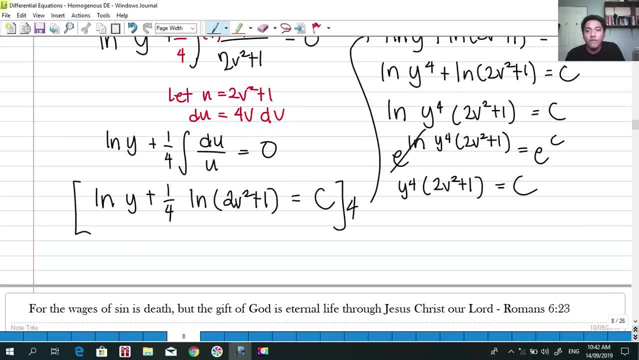 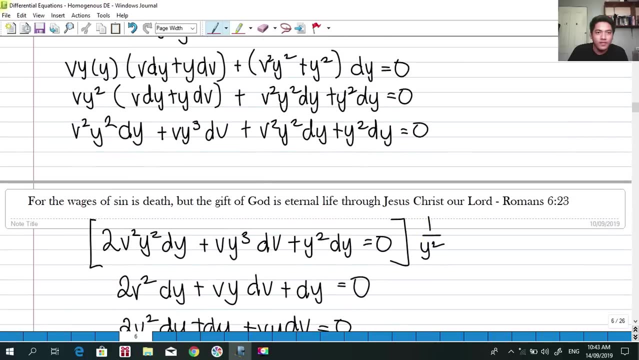 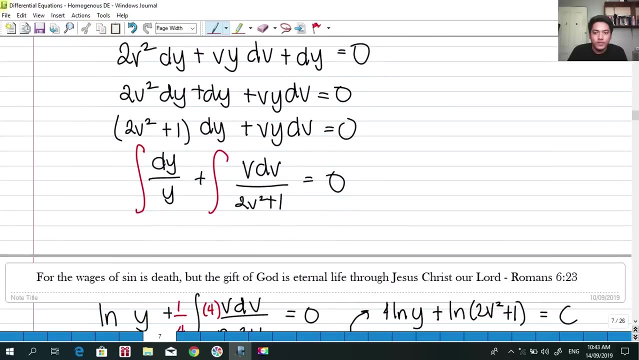 is this our answer? no, not yet, because it is in terms of B. so if we remember our substitution a while ago, we let: X is equals to B Y, if I'm not mistaken. let's just try to see it again. all right, X is equals to B Y. okay, X is equals to B Y, so 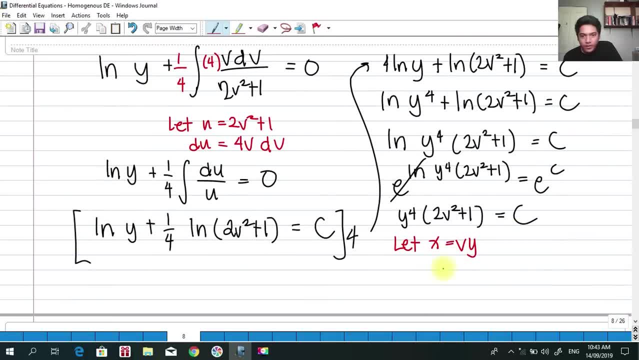 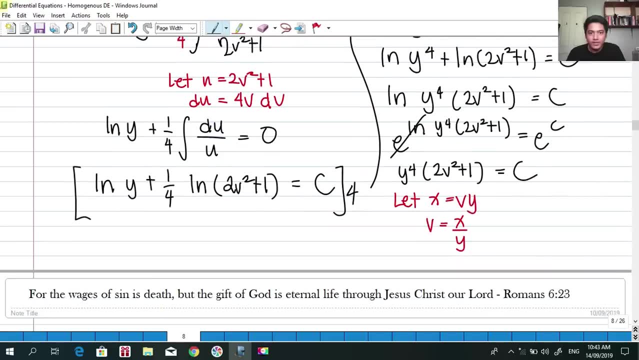 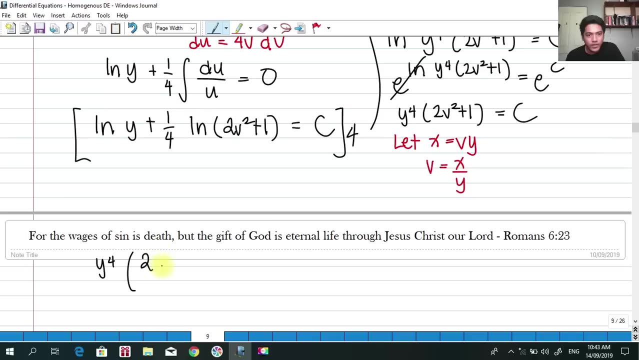 let's go back to our equation. so here B would become a X over Y because of this. so let's substitute it back with B. so we have Y raised to 4. okay, we have 2b squared. what is our B squared? so that is what: 2b. 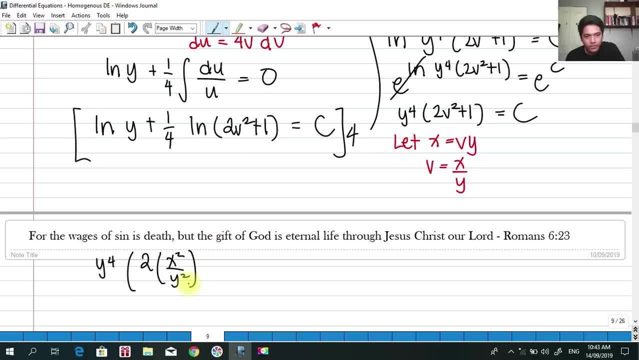 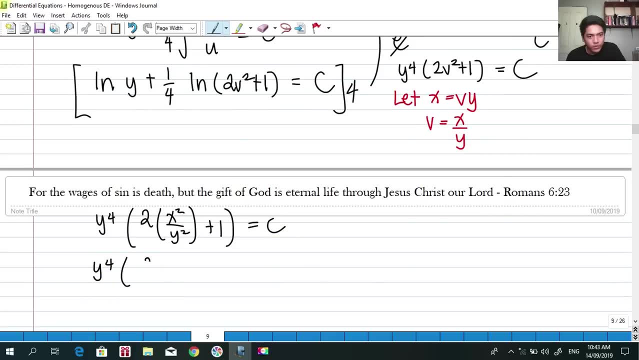 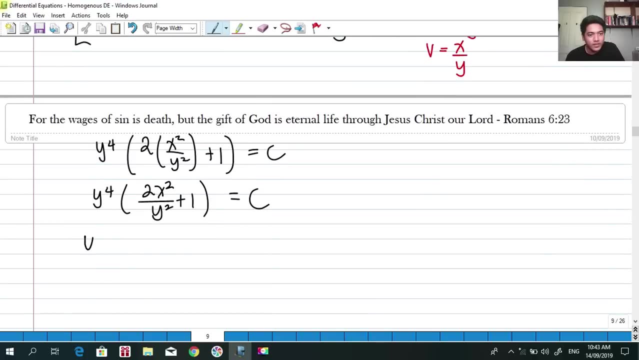 squared, we have X squared over Y squared. okay, plus 1 is equals to C. that is our 2b squared. so, simplifying: we have 2x squared over Y squared, plus 1 is equals to C. and further simplifying this, we have very y raised to 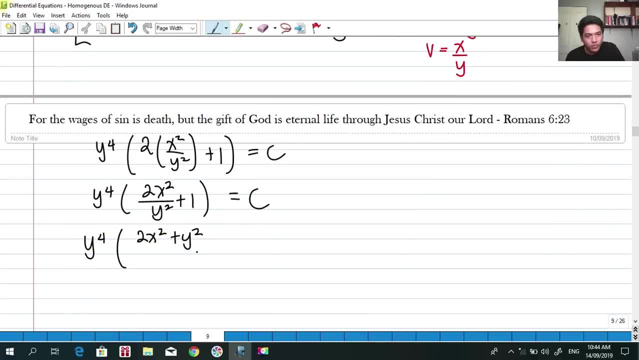 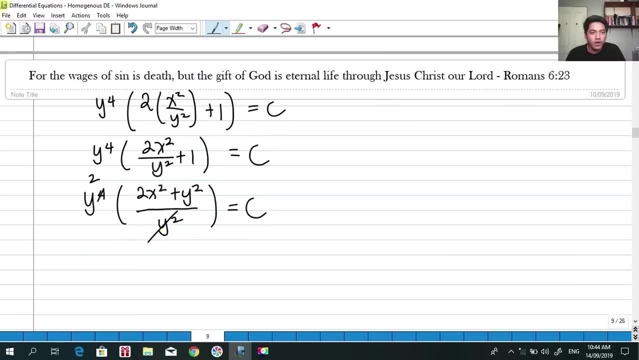 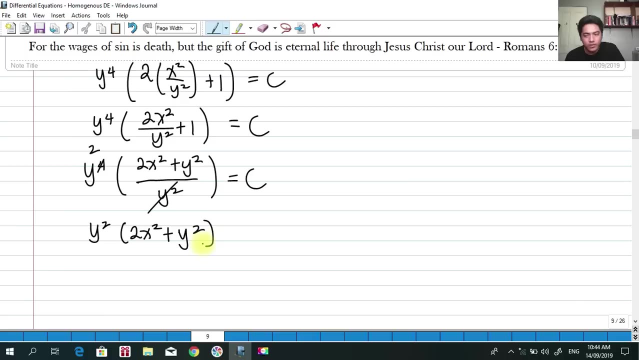 4. 2x squared plus Y squared over Y squared is equals to C, so we can see that this should cancel away and we are left with an answer of Y squared. okay. times 2x squared plus y squared is now equal to C, so this should be our answer. 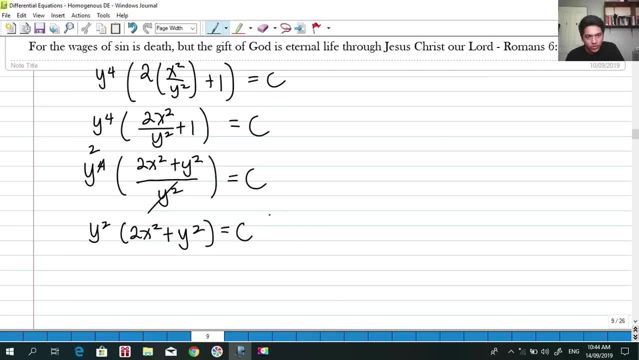 Our general solution for our differential equation. okay, So that would be our general solution. So what if I'm going to? this should be our general, okay. What if there is a condition? okay, This is an add-on problem, okay. 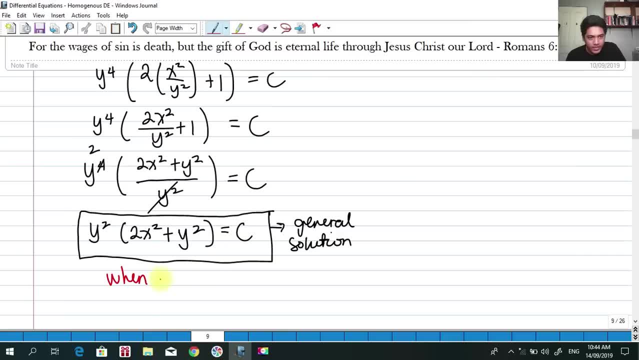 If there is a condition when x, let's say, is equal to 0,, y is equal to 1, okay, If there is a condition, as we all know in solving differential equation, if there is a condition, probably the problem is asking for the particular solution of the DE. 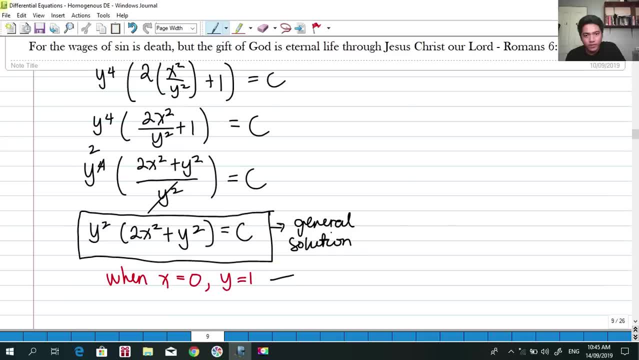 So, simply, we're going to find the value of c by simply substituting this value. So we have y squared, that is 1 squared Times 2 times 0 squared. okay, This should be 0.. Plus 1 squared, okay. 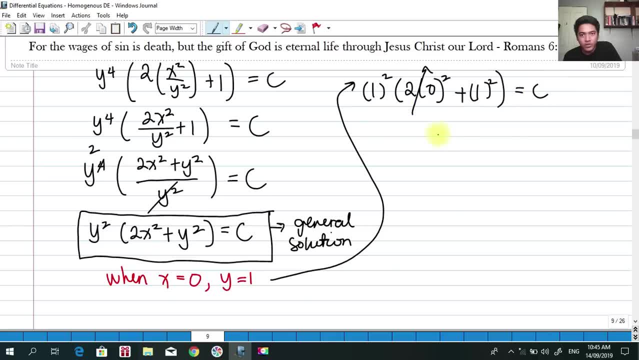 Is equal to c. As you can see, this should be 1, 0.. So our c is equal to 1,. okay, So, because 1 times 1 is 1.. So hence, our particular solution would be: y squared times 2x squared plus y squared. 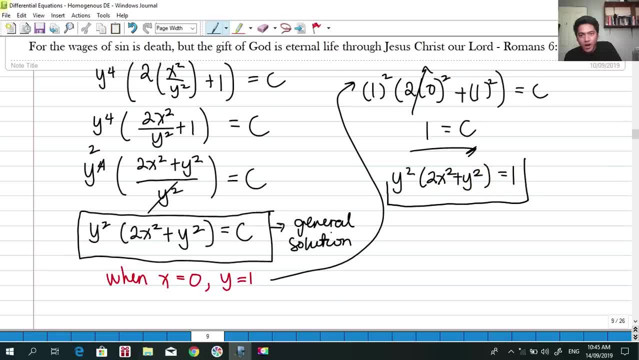 is equal to 1.. This should be our particular solution, Okay. So particular solution Okay.